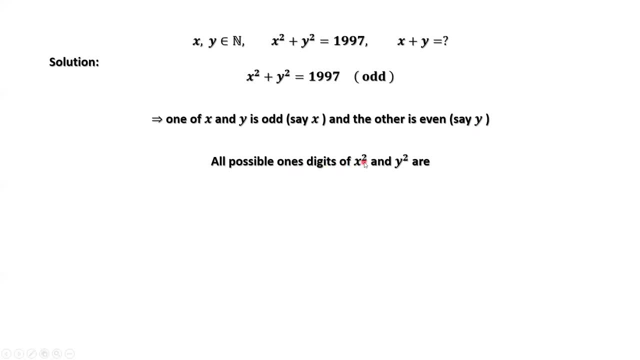 All possible ones. digits of x squared and y squared are 1,, 4,, 5,, 6,, 9.. This is a general result. If x and y are positive integers, x squared plus y squared equals 19,, 97.. 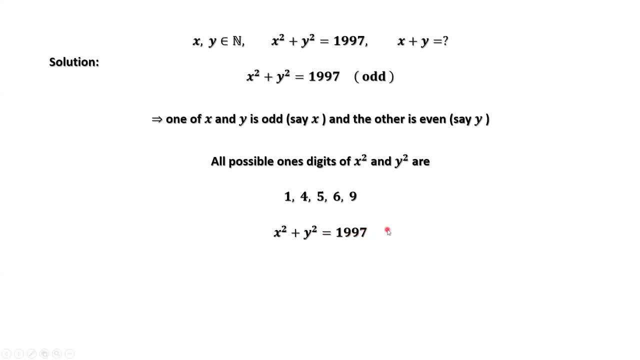 The last digit of 19, 97 is 7.. x and y squared have one digit of 1 and 6. All possible ones digits of x have odd numbers. The only possible combination for one digit of x is the result included. 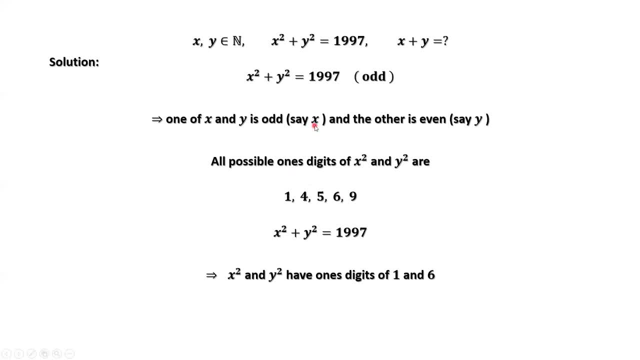 The falling number of digits to be divided by 5.. The only possible combination for 1 and 6.. The cold number of digits is 3.. What is the one-stitches of x? One-stitches of x is 1 or 9,. 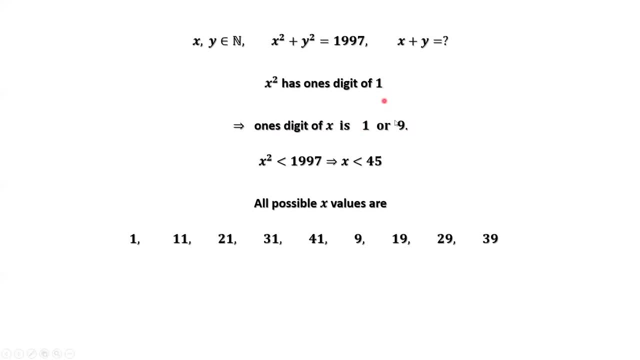 because 1 squared is 1.. 9 squared is 81.. The one-stitches of 81 is 1.. From the given condition, x squared plus y squared equals 1997.. Both x and y are bigger than 0.. 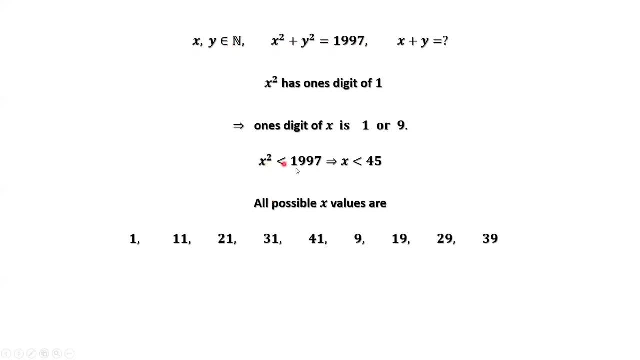 Therefore, x squared less than 1997.. Taking squares on both sides of this inequality, we have x less than 45.. All possible x values are 1,, 11,, 21,, 31.. All possible x values are 1,, 11,, 21,, 31.. 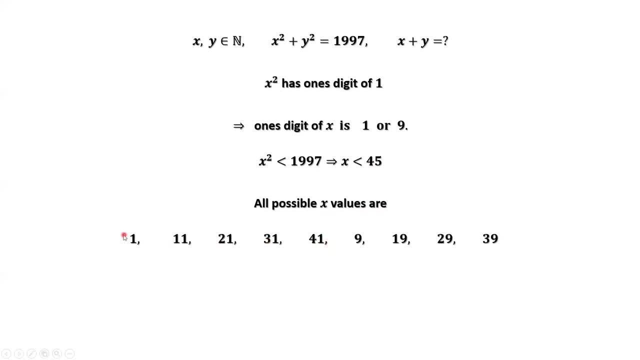 All possible x values are 1,, 11,, 21,, 31.. These numbers have one-stitches of 1.. These numbers have one-stitches of 1.. 9,, 19,, 29,, 39,. These numbers have one-stitches of 9..